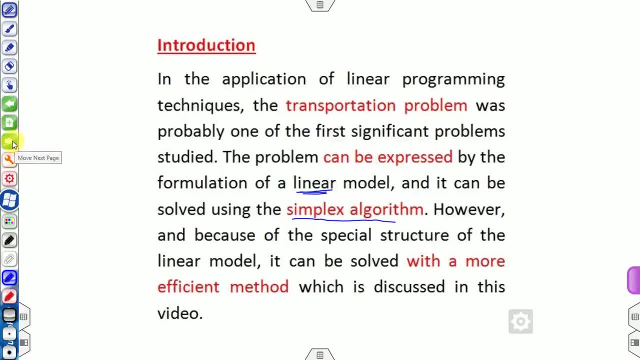 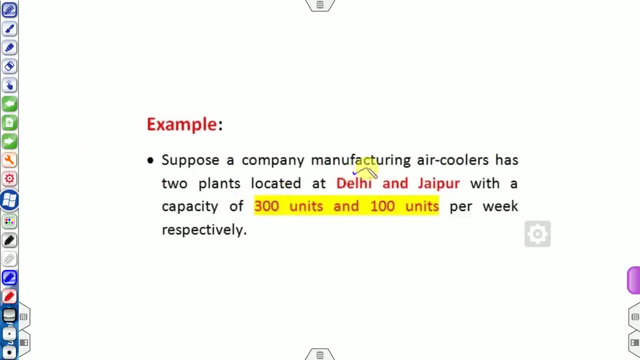 just explain the mathematical models and the terminology behind it. Say, suppose that a company manufacturing the air coolers that has the two plants stated at the Delhi and the Jaipur speed, which has the capacity of the three thousands and the three hundred and the one hundred units per week, Okay, 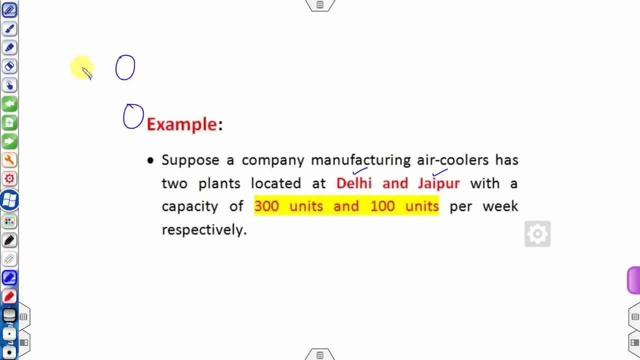 So it means I have the two units, that is, one is the Delhi and second is the Jaipur. Okay, They have manufactured certain products of the air coolers are there. So what is that? Once they manufacture that, then definitely they will transport their air coolers to the depth, to the 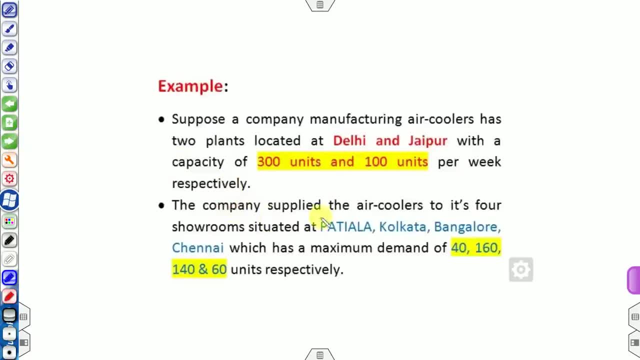 different stations. Okay, So the company supplies the air cooler to its four major showrooms are there. So, for example, this one showroom is in Patiala, second is Kolkata, Bangalore, Chennai is there, And the maximum demand for this Patiala is 40 units. 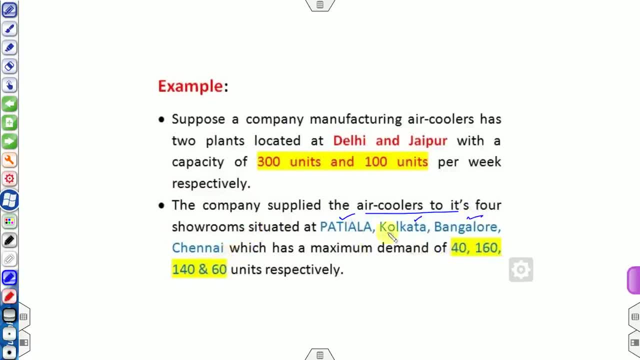 Kolkata is 160 and 140 and 60 for the Bangalore and Chennai respectively. So what will happen? Since the Delhi has the different raw materials, different man powers, are there different working and all other conditions. Similarly for the Jaipur also, they have the different man powers. 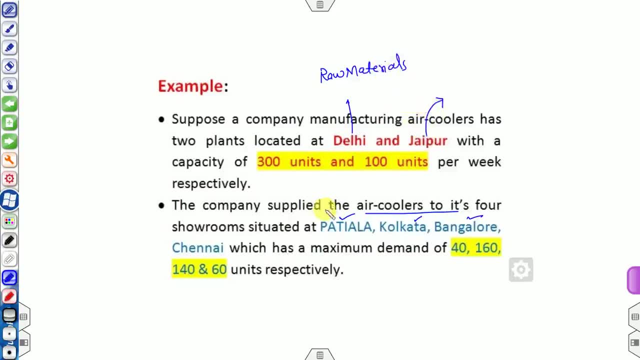 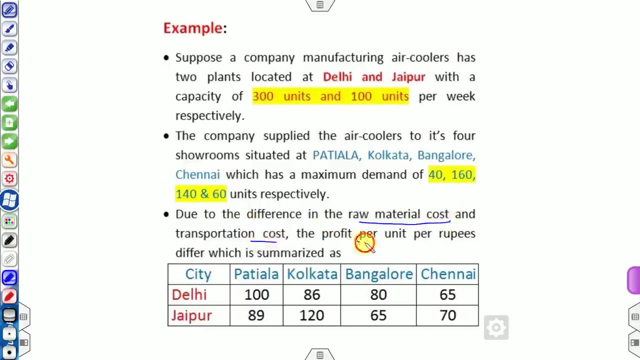 they have the different raw materials and so on. So definitely there is a technically slightly change in their air coolers. models are there. So what will happen? So, due to the difference in the raw material cost, transportation cost the profit per unit. 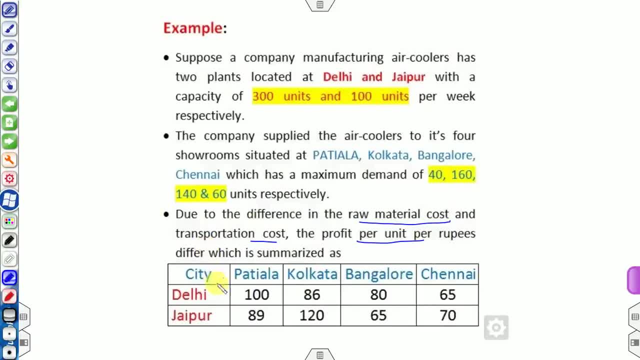 per rupees differ, which are quite obvious- that, for example, the air cooler which are designed in Delhi and transport to the Patiala, the profit will be 100. While similarly, if the air cooler which are manufactured in the Jaipur plant they transport to the Patela, then the profit will be 89. 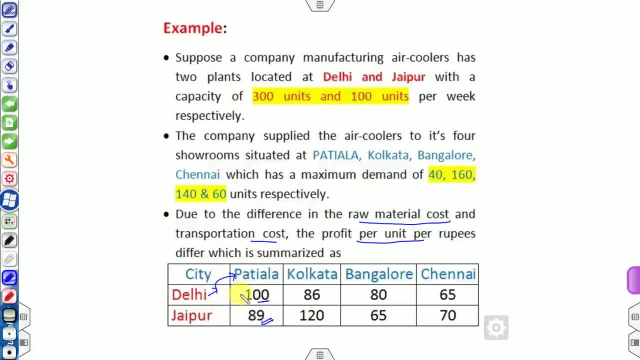 it's quite obvious, because Patela is near to the Delhi, so the transportation cost is less as compared to the Jaipur. so the profit will be highly similarly for the Delhi to Kolkata, Delhi to Bangalore. and these are some profit per unit, per rupees are there which are definitely differ? 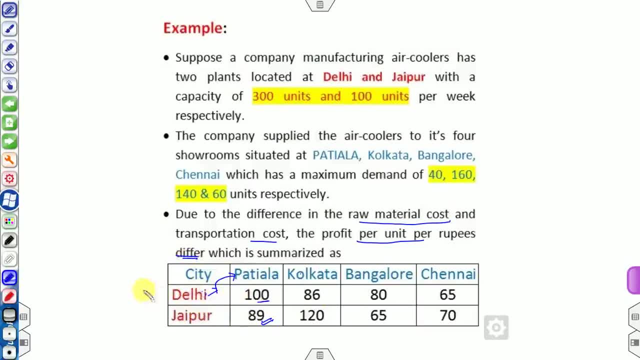 from city to city and from the manufactured plant. so the question arises: is so what is that? the daily capacity of the Delhi is 300, so maximum they have to 300 units be product. for the Jaipur they have the maximum 100, while for the Patela the maximum demand is 40, while 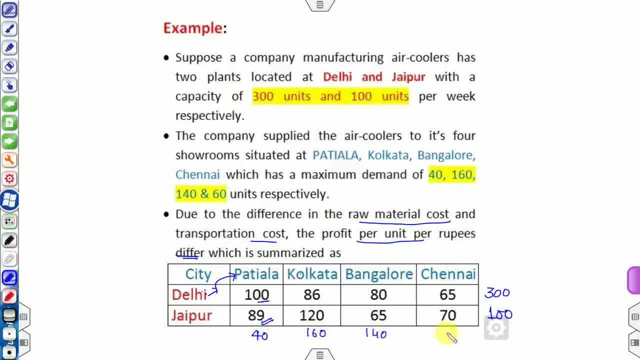 for the Kolkata is 160, Bangalore is 140 and here is 60. okay, so what is the meaning of them is, the Delhi has the maximum of the 300 air coolers and the Patela restriction is 40, the maximum 40 air cooler. they can buy them. so from where they can buy, either, they can buy from the Delhi. 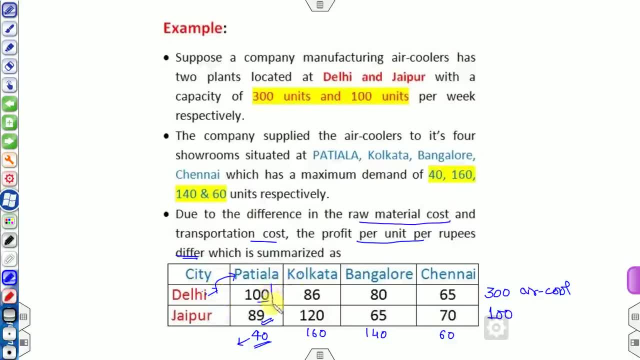 or from Patela. it may be that he can buy 40 unit directly from the Delhi and there is no unit buy from the Jaipur. or he, or, or they can buy 20 units from the Delhi or 20 units for the Patela, okay, or? 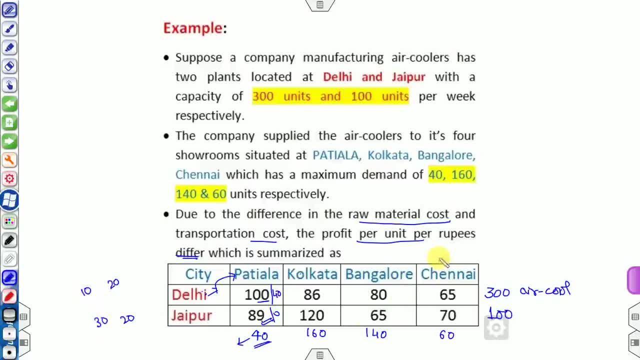 any other post, any other combinations are there: 10 and 30. for example, and on the other hand, if the Patela by the 40 units directly from the Delhi, it means the remaining 260 units are distributed among the Kolkata, Bangalore and the Chennai, while 100 units are completely. 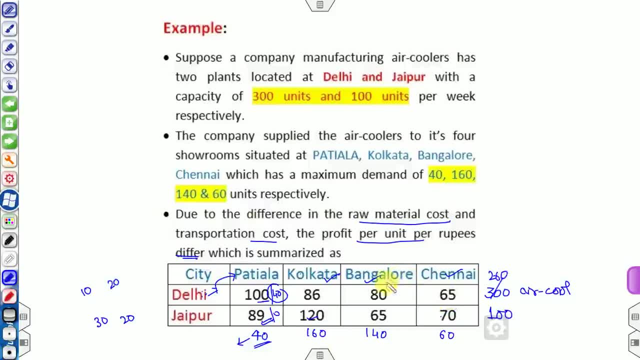 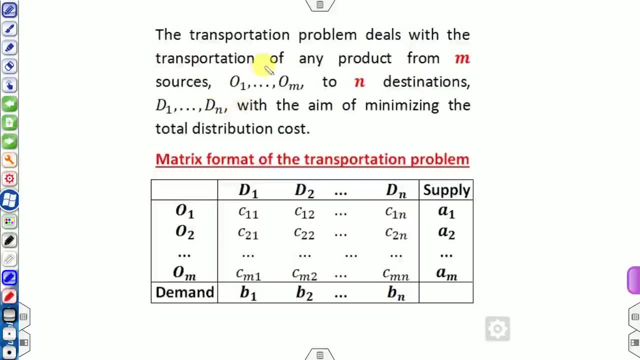 distributed in these products. so such type of the models can be formulated with the help of the transportation. okay, so in in general. so if I say there are the here, in the previous case there are only the two sources: one is the Delhi, second is the Jaipur. so in general, if I say there, 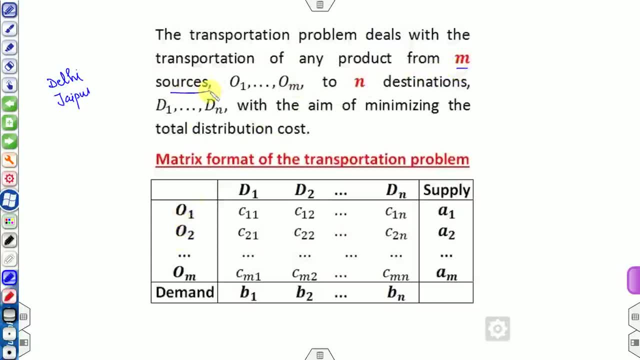 there are my M sources. These are my M sources. So here are my sources. Okay, O1, O2 and up to the M sources are there And their target is to transport their products from the one source to the destinations are there. So here I just consider, there are the M? N number of the 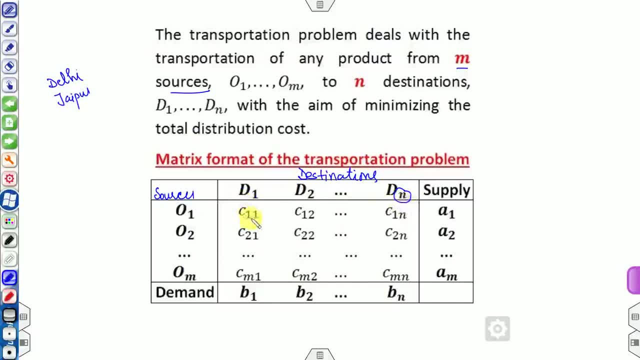 destinations are there. Okay, And what is the C11?? That is a cost. What is the C11? is the cost, that is, the transportation cost of the source one to the destination one. Okay, That is a C11.. Transportation cost that is being from O1 to the C1.. Look at the previous one. 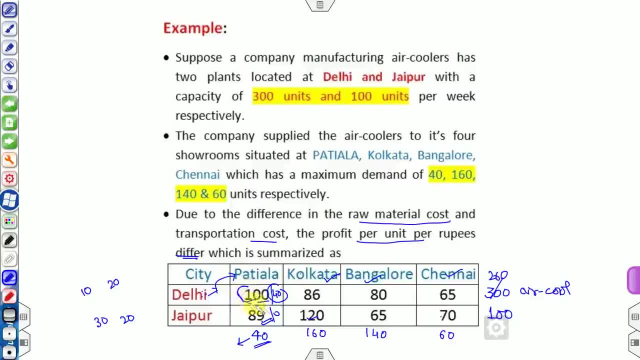 This is my C11.. Okay, That is 100 C11.. So C11 means that is nothing, but C11 is means you have to transport the cost from the C11 to the destination one. Okay, So C11 means that is nothing but. 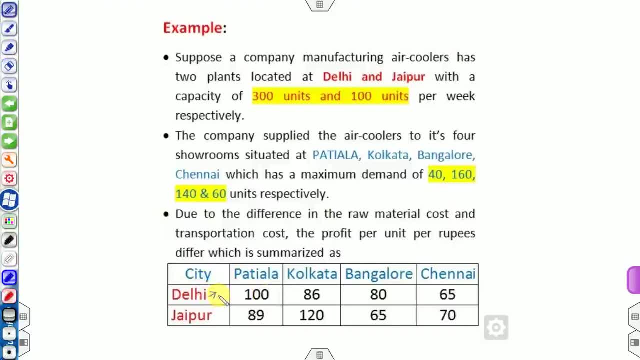 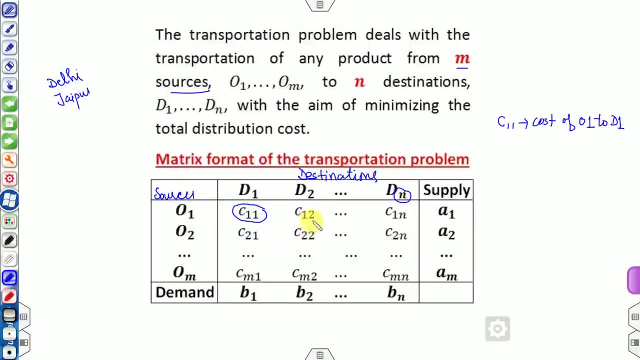 city, from the plant Delhi to the city Patialapur. Okay Now, similarly, C12 is the transportation cost of the source O1 to the D2, and so on. Here, A1 represents the maximum supply by the source O1.. A M represent the maximum source of the O M, And this B1, B2. 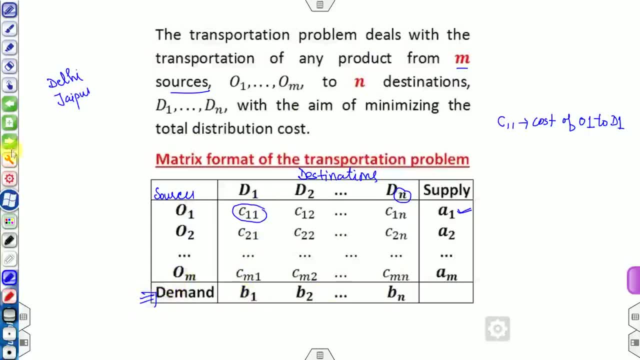 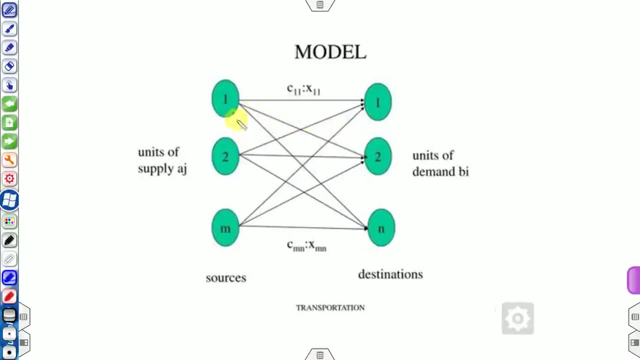 they are representing the demand. So this is the matrix formula. because this is the matrix formula, So this is the matrix formula, because this is the matrix formula is representing in terms of the matrix. are there? So how many variables are there? total in this format is MN. Okay, So, in order to represent in the model form. So if I just 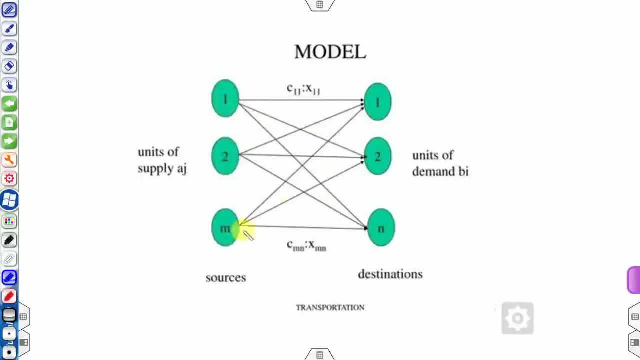 consider: these are my sources: M01, O2, OM, OM and these are my destinations. are there and each source can. each source can send their products to each destinations are there. So I'm going to name the one source: M01, O2, and so on up to O, and are there. So when the one 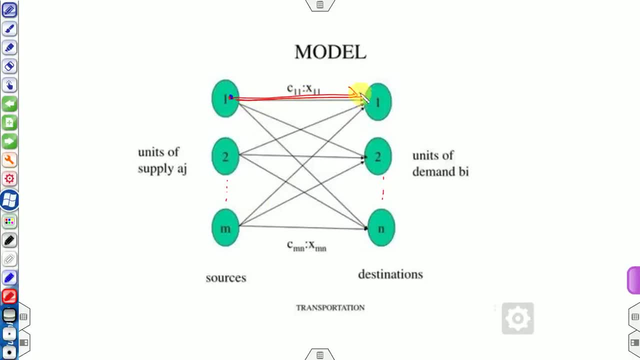 source O1 transport the units to the destination one. that transportation cost is C1.. Okay, Here X11 represents the number of the products transferred. Okay, So I know that there's a transportation cost from one source to the one destination, C1.. So the question arises. 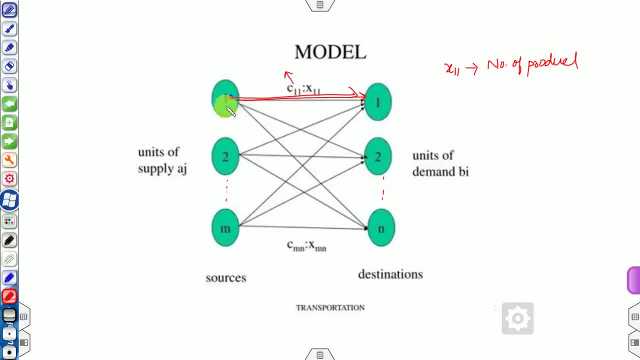 how many units we can transfer or we can transport from the one source to the second source is denoted by x1.. So, in general, I call, as xij is representing my number of the units, that is transport: number of the units: transport from ith source to the jth destination. Okay So, and similarly, cmn is the cost when you. 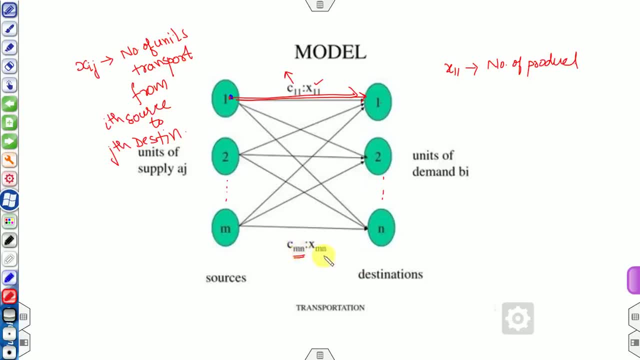 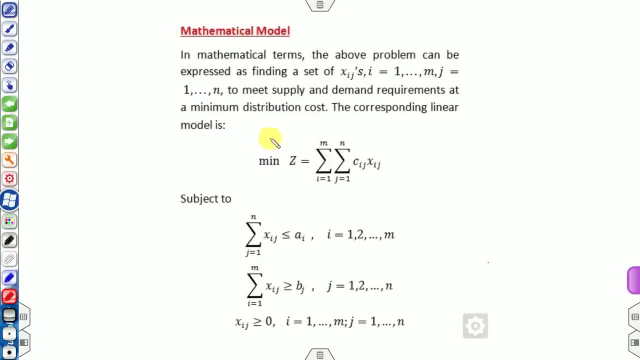 transport from the m source to the nth destination, and xmn represents the number of the units we can transport in such case. So based on it we can generally define, because our target is to transport the products b. So definitely, when you transfer from product a to b, there is a cost, cij, and your target is to minimize the cost. 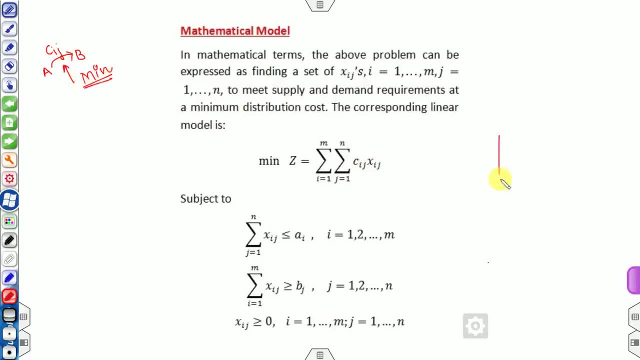 b. Okay, So what will be the total cost? b. So if I say this is my c11, this is my c12, and so on and up to cm1 and cmn, Okay, So when you transfer, when you transfer one, when you transfer, say, x11, 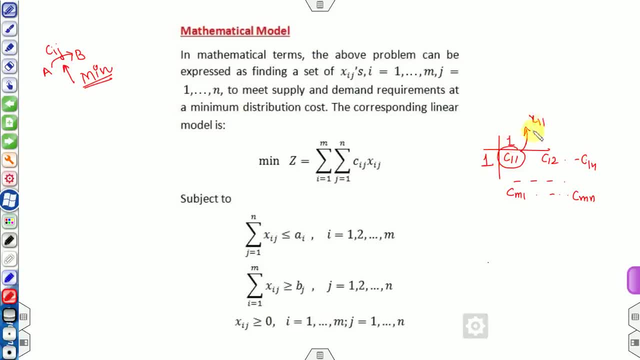 products from the source 1 to the destination 1.. So when you transfer, say, x11 products from the source 1 to the destination 1. So the cost will be c11.. So the total cost will be c11- x11.. Similarly, the cost for transfer of 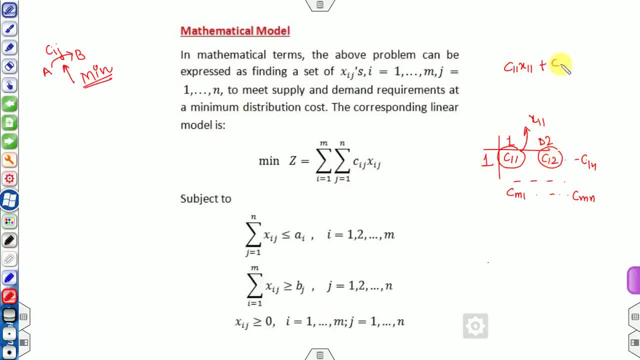 source 1 to the destination 2 is c12 and I assume that there are the number of products are x12.. So the total cost will be this one. that is, this plus this and up to last one is cmn xmn. So what are the restriction on that? that is the maximum source here. look at that, the maximum source. 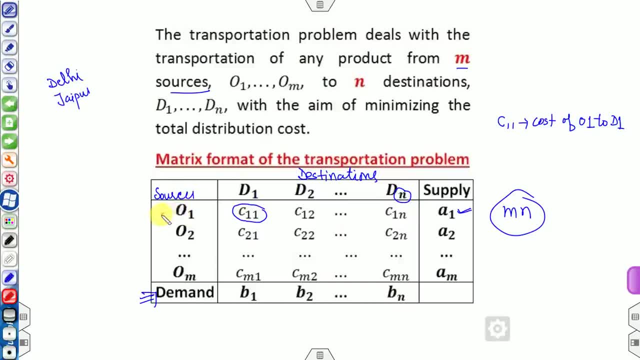 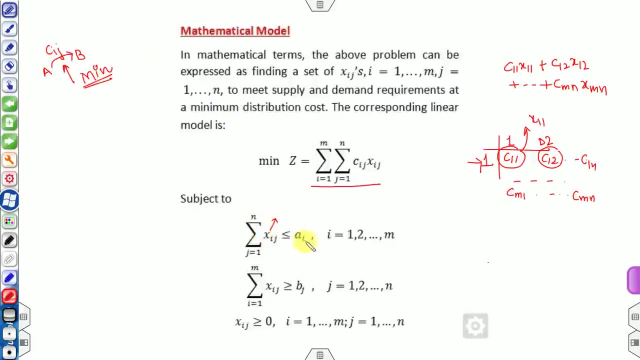 of this here. the maximum source of o1 is a1. the maximum supply of the o2 is a2. this is the maximum supply. Okay, So it means the constraints are you have to provide supply x11, x12 and so on, which is: 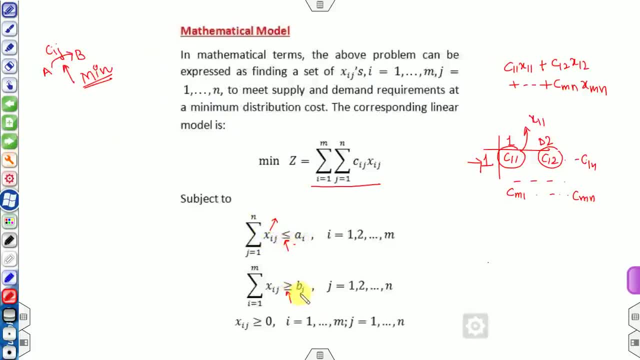 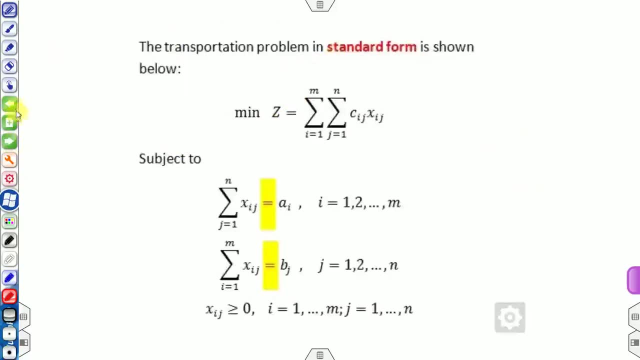 the less than of this and second for the greater, because this is the demand is there and xij are greater than 0.. Okay, So, since this contains the, some inequality or equalities are there. So when you transfer to the standard form, So 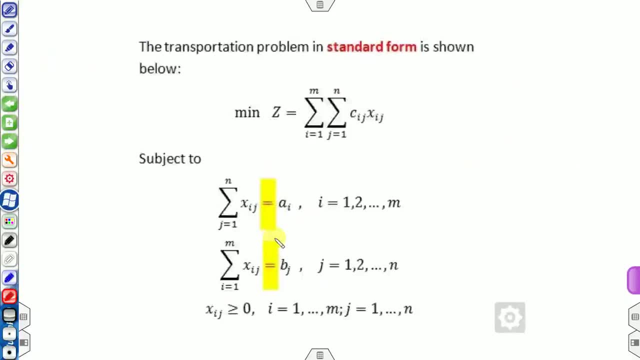 nothing, but there are equality signs. are there, including slacks or plus artificial, or whatever? is there? Okay, So that is the minimization of this, and so on. So now, when you know that this is the standardized form, So you can solve it with the help of the simplex method, dual simplex. 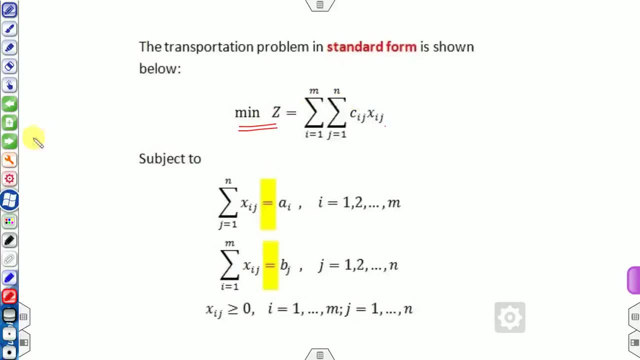 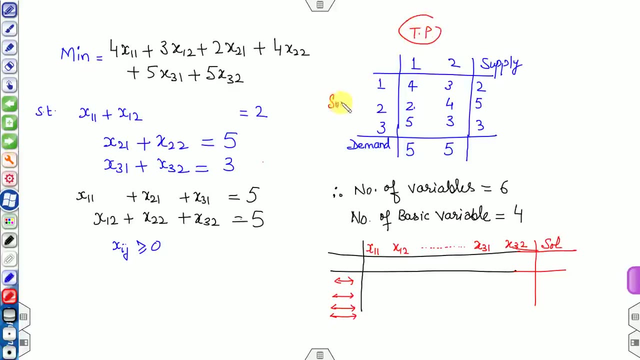 method, graphically or any other methods- are there, But what are those drawbacks are there? look at that just. I just consider this as a transportation problem in which I just consider as a full three sources and the two destinations are there and four, three. these are my cost, Okay, And these. 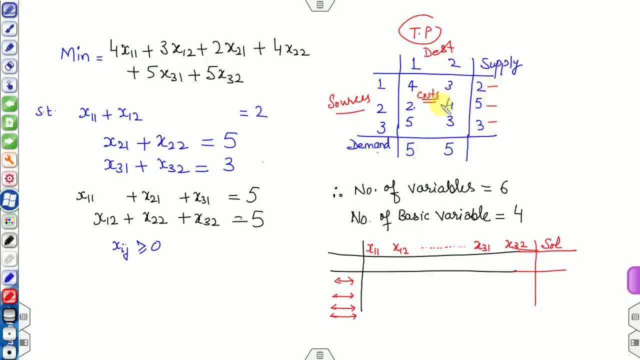 are my supply, this is the maximum supply and these are the demand of the destinations. So look at that. what is the objective function is c11, that is four. number of the unit we can transfer from the one to one is 11.. So 4x11 plus 3x12, plus this, this, this, this. So this is my objective function. 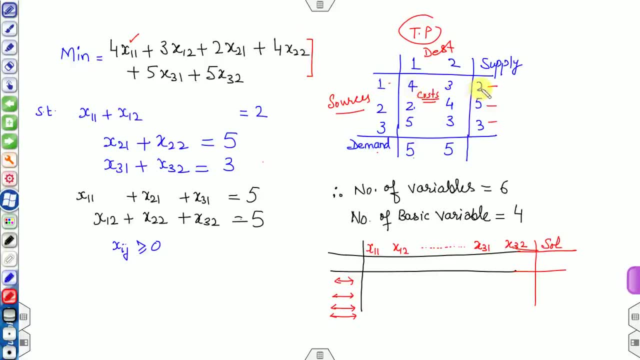 What is the constant is 4x1, because this two, that is, the supply of the source, one is two, can be split up either as a here or here, or both of them. that is 111.55 and so on, So that constant is x11. here's the number of the. 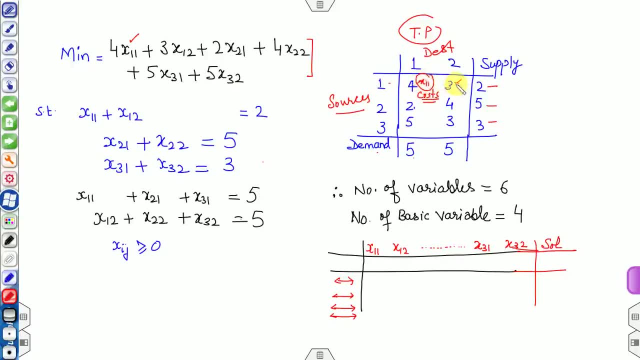 units you have transform is x11.. So x11 plus x12 is equal to 2p. similarly, for the second: x21, x22 is 5, x31, x32 is 3.. Similarly for the second: x21, x22 is 5, x31, x32 is 3.. 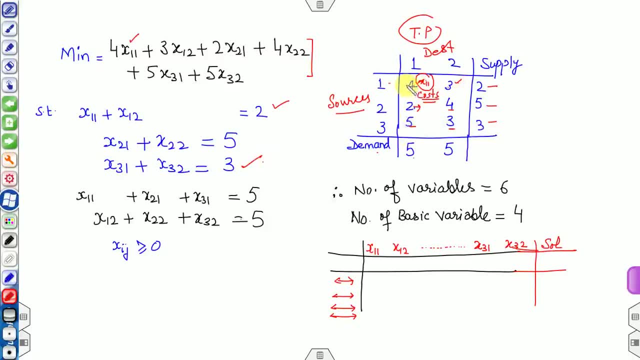 Similarly for the column wise: this is my x11,, this is my x21, x31.. So x11,, x21, x31 is nothing but the 5.. And similarly for the others are there. Now, when you try to solve this with the: 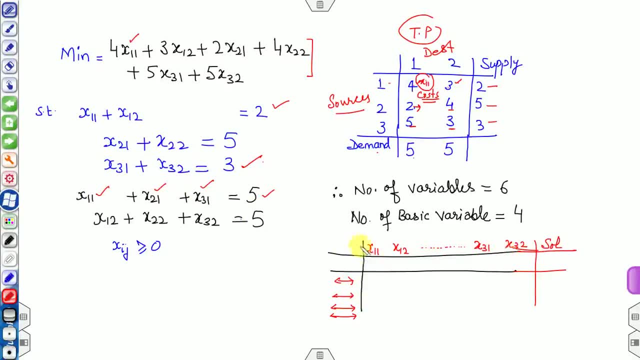 help of the simplex method. so look at that. how many variables are there? So x11, x12, up to the x32. And other slack or surplus are there. So when you try to solve, this is there. So these are there. So look at that. how many variables are there in this simple example? 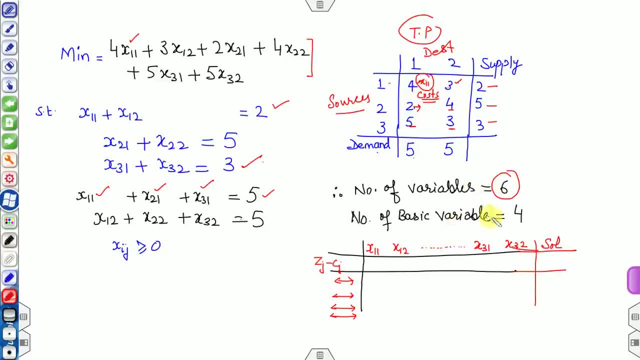 that is a 3, cross 2, that is a 6 are there, And number of the basic variables are 4.. So this I just calculate here as m plus n minus 1.. Here m is the number of the rows. 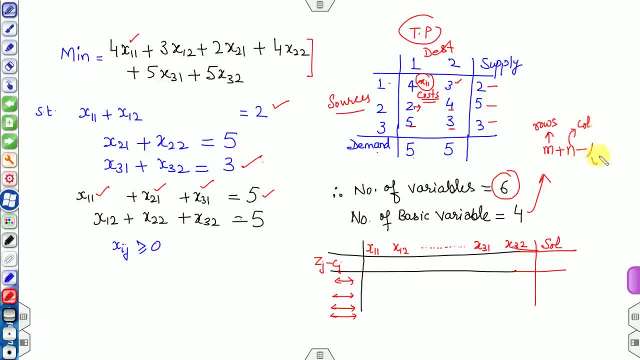 n is the number of the columns and n1 is there. So 3 plus 2 minus 1, that is nothing but the 4. Or otherwise, when you substitute here, look at that x11, what is the column of the x11 is 1, 0, 0,. this is 1 and here is 0. 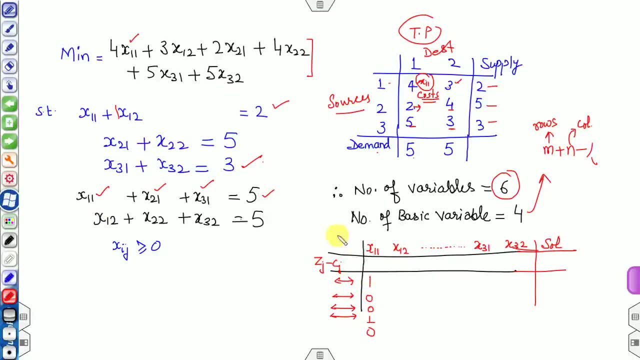 Similarly, what is the x12?? Here is 1, this is nothing. this is 1, this is nothing. 0, this is nothing 0, this is nothing 0, here is a 1, and so on. So look at that, the problem is. 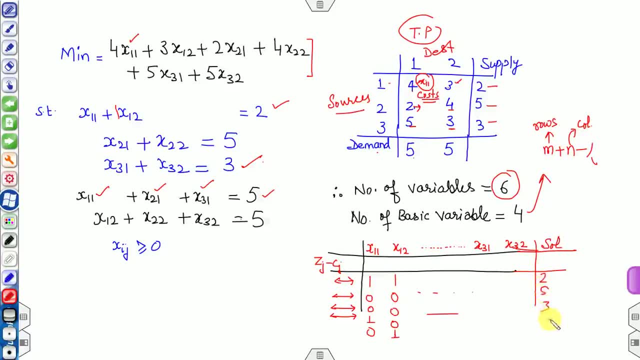 very complicated, very complex, is there? Okay, And so on. So, in either case, you have to find, firstly, this, and so on. Also, we can see that, since all are the equality signs, so from here you can find the value of the x11.. So what is the x11? 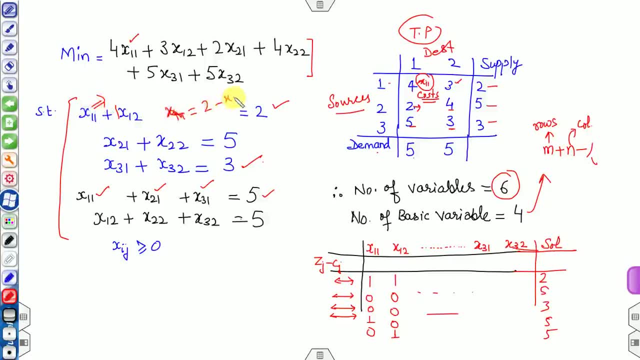 is So you can find it as 2 minus x12 and you can substitute here Okay And so on. So that is why this is a very lengthy method. So in order to solve it, there is some methods, which is involved. 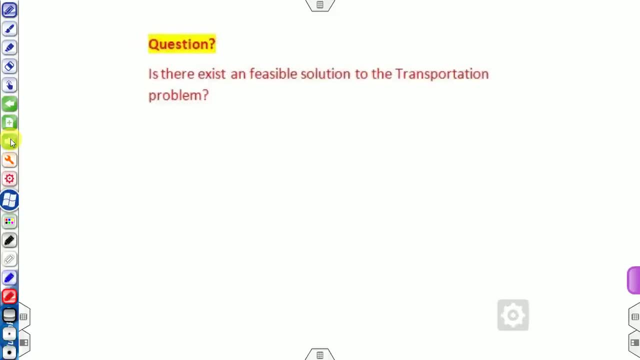 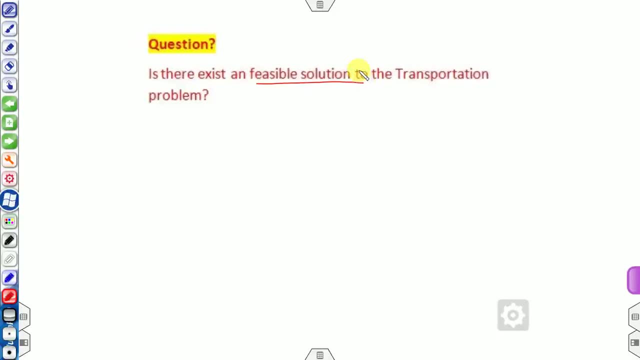 solution exists to the transportation problem. Remember we are not talking about the optimal solution. Firstly, because optimal solution occurs when, when there is at least one feasible solution. So first question arises, obvious that is there any existence of the feasible solution in the transportation problem? If my problems are look like, say this, this is my problem. 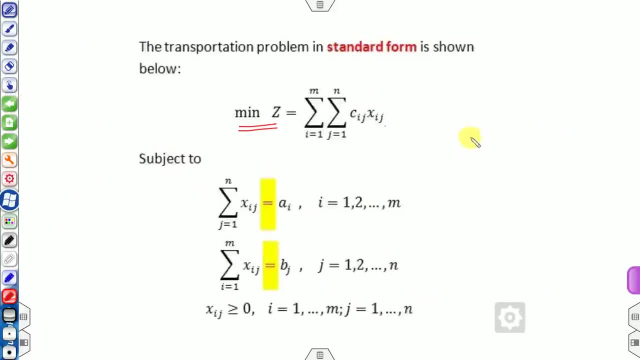 okay or this is my problem. So, whether there is existence or check any feasible solution or not, Because if there is an existence of a feasible solution, then we may try to move on the optimal solution. If optimal solution exist, then it is okay. 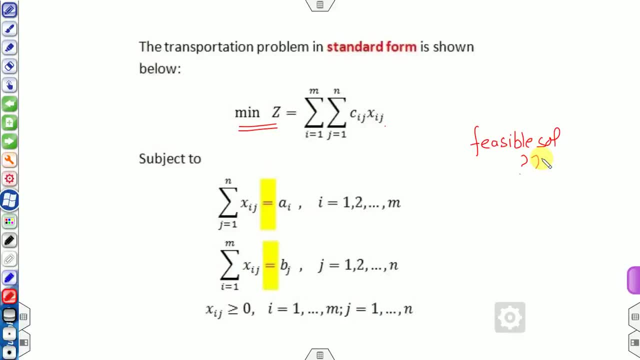 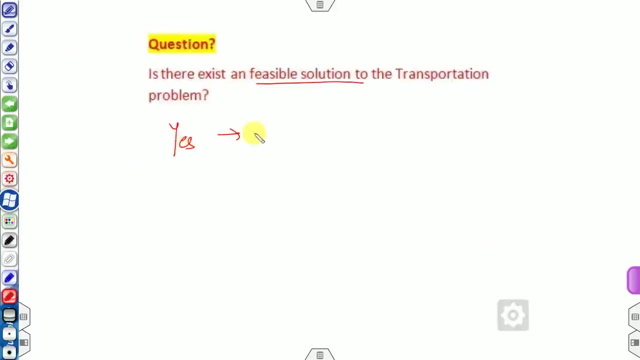 If optimal solution does not exist, then we call it as the unbounded solution. So here the question arises that if optimal solution exists, if the answer is yes, then under which condition? Okay. So first thing is that when the officersal, which is the right answer, since x11 and x12 are possible conditions d now and this time Just to apply this мик, you need to check whether any reasonable and applicable solution exists, and if it exist, then under what conditions. Okay. So first thing is that when the 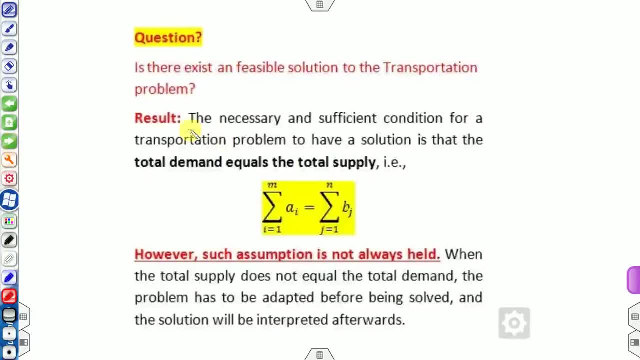 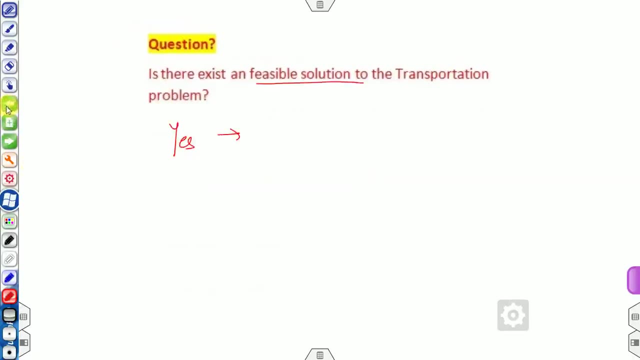 optimal solution, when the feasible solution exists, is that the answer will be here, the necessary and the sufficient conditions for the transportation problem to have the solution is that total demand is equal to total supply, this one, okay. so look at that if i say, if i just consider this example. 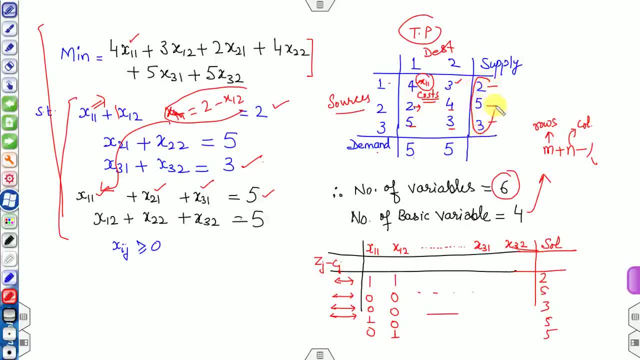 this is what is the total supply. is that is a sum? that is my 10. what is the total demand? is again 10, okay, so if both are equal, then there is a guarantee- remember, student, there is a guarantee that at least one of the solution is the feasible okay. so look at that. this is the feasible okay. 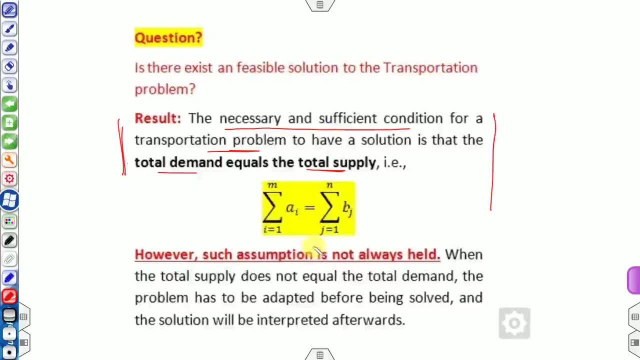 but remember that such conditions may not always be hold. for example, for a very recently, a lockdown period is there be? so what is that? there is a huge demand, but the supply is less. okay, so there is a huge demand but supply is less. on the other cases, in the normal days, it can also be. 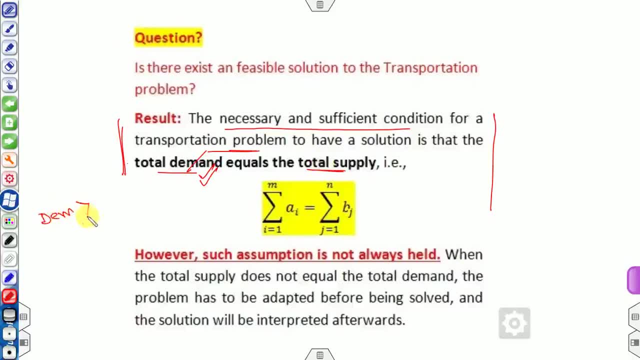 there. sometimes the demand is very large as compared to the supply, okay, or sometimes the demand is very less, but supplies the huge one, okay. so in such case, so such case, there are the two cases. one is that when, whether the this constraint satisfied, or either this constraint. 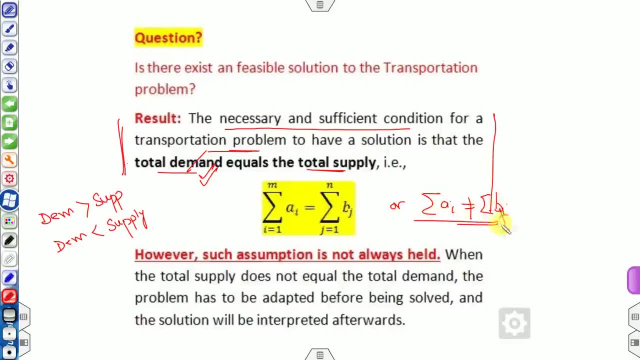 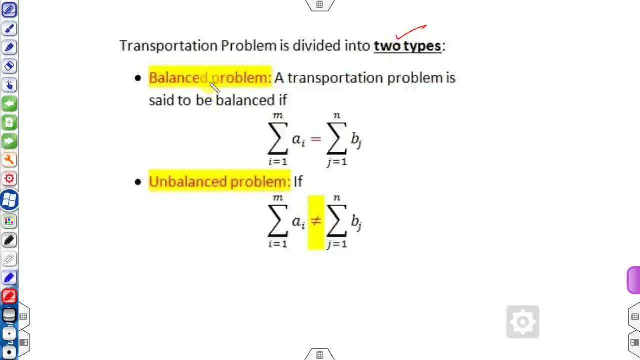 violates that, okay. so that's why we just discretize the transportation problem into the two types. one is the balanced transportation problem, second is the unbalanced transportation problem. so balance when the source, when the total supply, is equal to total demand, okay. and on the other hand, unbalanced problem when the supply is not. 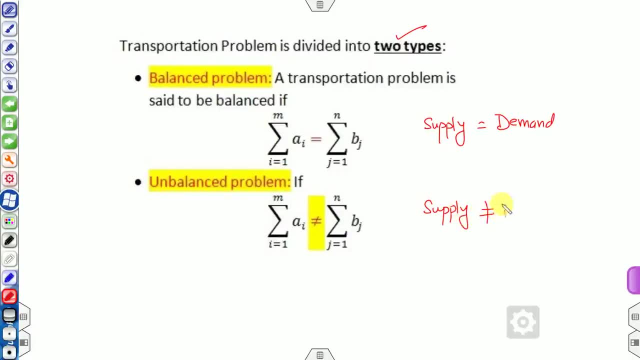 equal to the demand. remember this is: the total supply is not equal to total demand. so when- remember whenever you are trying to solve the transportation problem, you have to firstly convert the unbalanced transportation problem into the balanced transportation problem, always, otherwise there is no guarantee for the feasible solution. remember the last slide here there is: 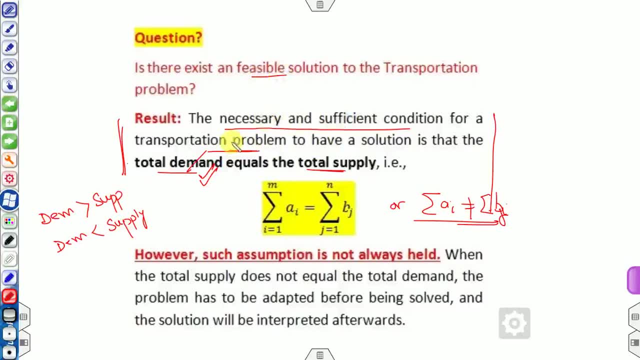 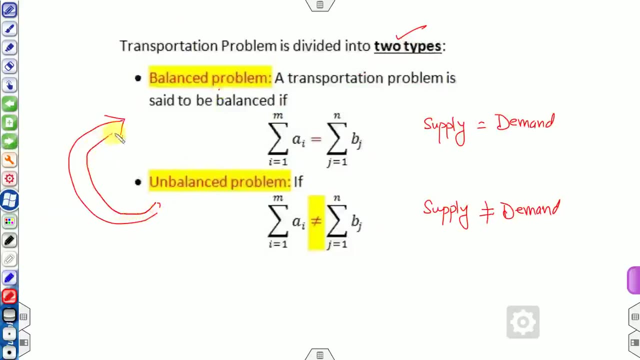 existence, to here the necessary and sufficient condition, only when this satisfied, and what is the condition for that? this satisfied when? if this satisfied, it means the problem will be a balanced one. so always, whenever there is an unbalanced problem, you have to convert into the unbalanced problem, you have to convert into the balance one. so how you convert them. so look at. 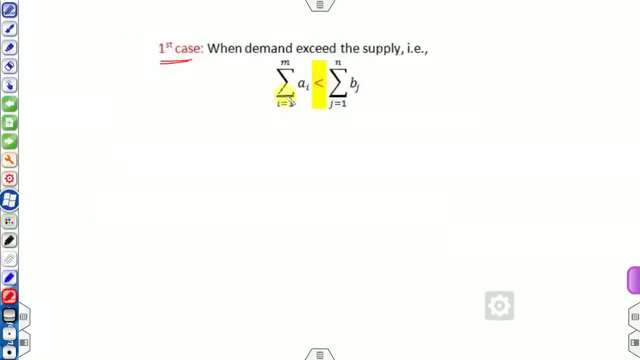 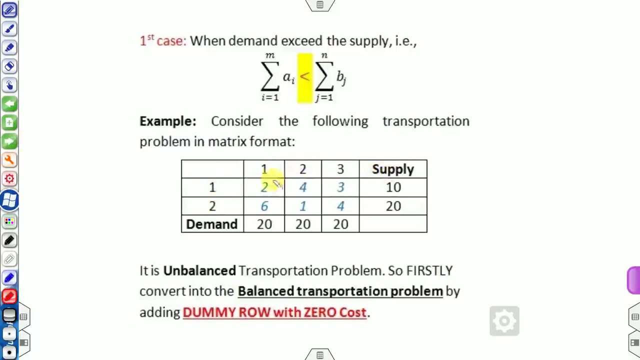 that. so there are the two cases. the case one when the demands exceed the supply. okay, that is, instead of the equality sign, it's a strictly less than sign. so what will happen? so look at the counter example. so assume that there are the two sources and the three destinations are there, and look at 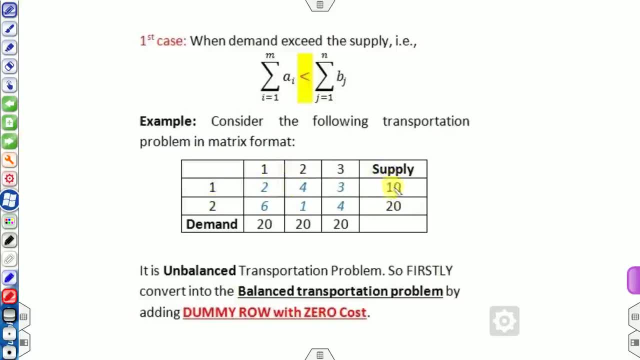 these are my cost: two, four, three and our supply. so look at what is our total supply. total supply is my 30. what is our total demand is 40.. okay, so clearly the 30 is not equal to 40, so it means this is the unbalanced transportation. 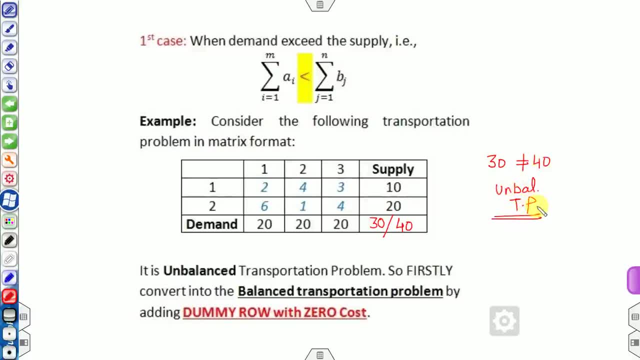 problem. so this is the unbalanced transportation problem. so you have to convert into the balanced transportation flow. so how you convert them: look at that: this is a 30, this is a 40, so there is a need to add the one extra row. okay, so there is a need to add the one extra row with the supply: 10. 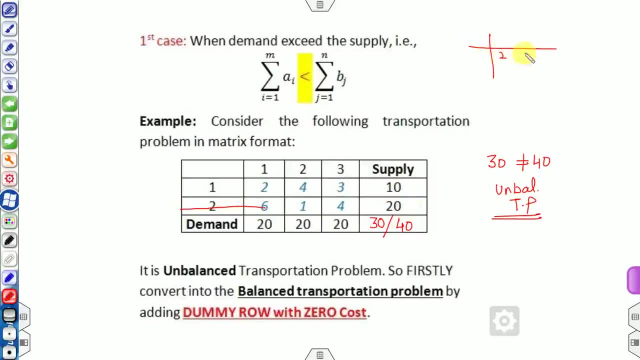 okay. so it means so far you have the two rows two, four, three and six, one, four okay, with the supplies 10 and 20, while the demands are 20, 20 and 20.. so there is a need of adding one extra supply. whose supplies of the 10 unit. but what about the cost? 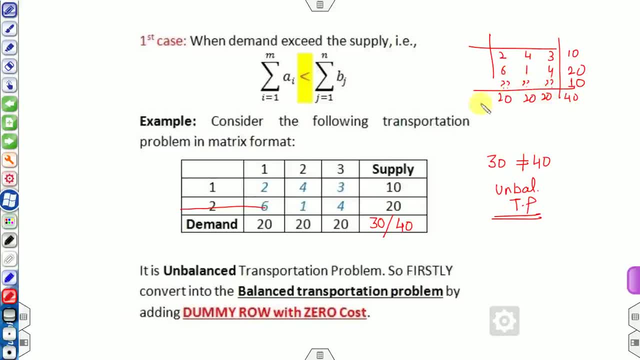 okay, so the cost is totally depending upon them. if you add the another supply, it means you have to add the another source, or three, but there is no source of them. so that's why, whenever you are trying to convert the unbalanced problem to the balance, firstly convert the, firstly converting to the 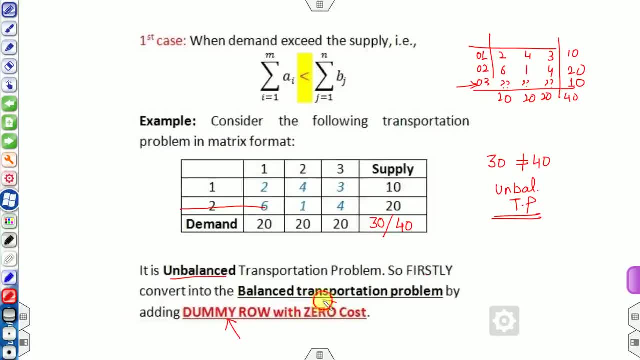 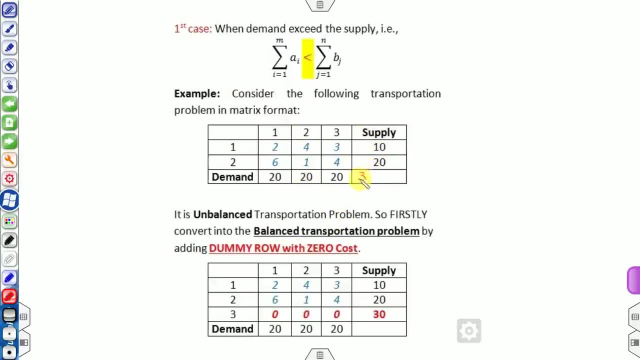 balance problem by using the dummy row, by using the zero cost. what is the meaning of that? look at that. that is this. this is the original problem. this is my 30, this is my 40, so you have to add the um uh dummy row. this is called as the damir. okay, with the zero cost. 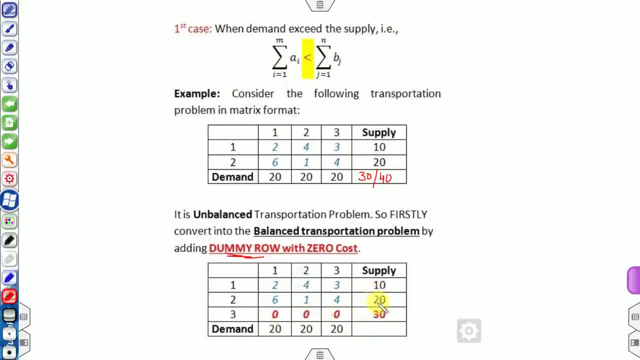 while the supply is 40. now it will be. look at that. so sorry. uh, this is not. yes, it's a 30. okay, so it's a 30. so you have to add: this is into balanced one, so it will be. now it's the it's here. look at that. support: it's a 60. so again, here is a 60. so now it's. this is the balance one. 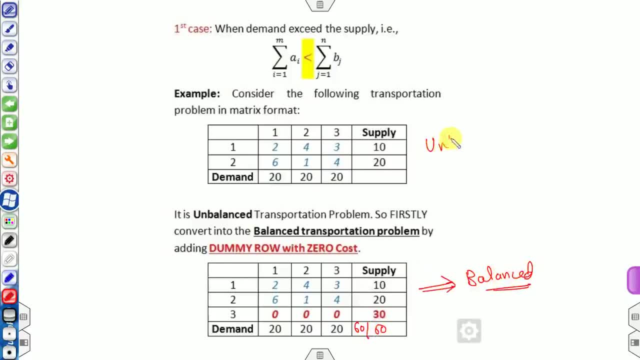 okay, so looks about 30.30ww0atm. camera is 30.60. always remember, whenever there is an unbalanced problem, you have to convert into the balanced problem by using either a dummy row or the column. look at the second example. so when the supply 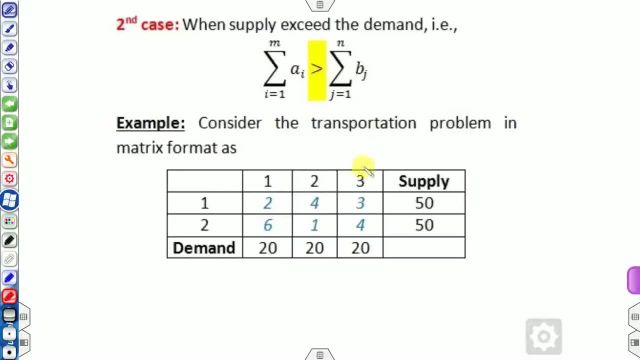 exceeds the demand, okay. so when this one is there, for example here, look at that. what is? the total supply is 100 and here is my 60. so again, this is not equal to. so it means this is my unbalanced problems. so what will we do? so you have to add 40 here. so you have to add another destination whose? 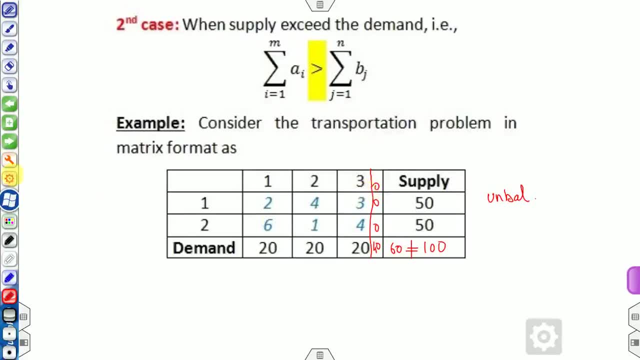 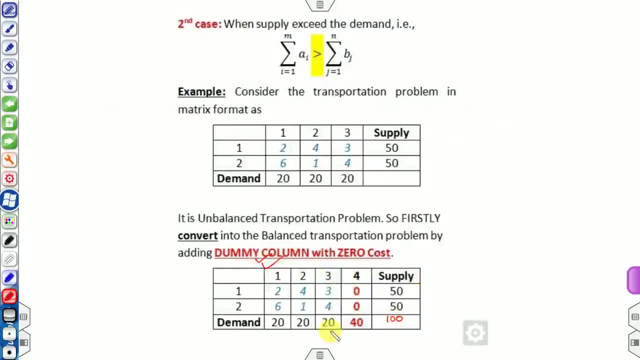 value is 40 and the causes are 0. so again, the look at that. this. you have to add another destination. that is a dummy column. now, this is 100 here. and look at that, this is again 100. so again, this is my balanced one, this is my unbalanced, okay, so i again repeat that whenever you are trying to solve. 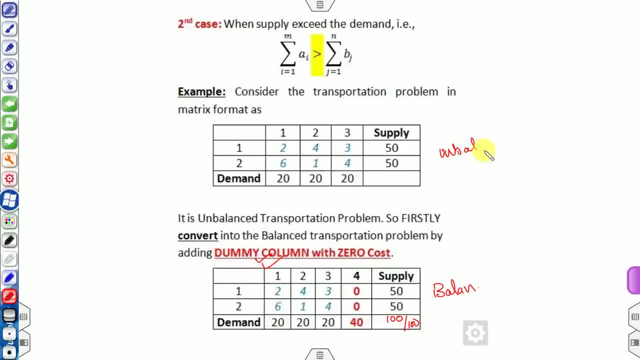 the transport, any transportation problem. the first task is to convert the unbalanced transportation problem into the balanced transportation problem by adding a dummy column or by a dummy row, according to that whether the supply is less than of the demand or greater than of the demand, okay, so. so what is the 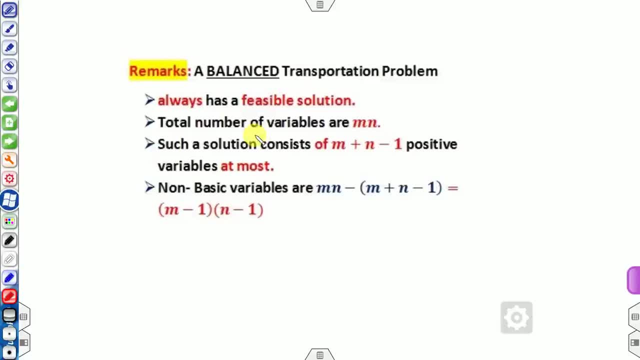 remark of that, because this uh talk is about only for the introduction. that is, the basic things are there, so remember, i just found the balance. so whenever you try to convert the unbalanced transportation problem into the unbalanced transportation problem, you have to add a dummy accordingly. so remember, i just found the unbalanced transportation problem. 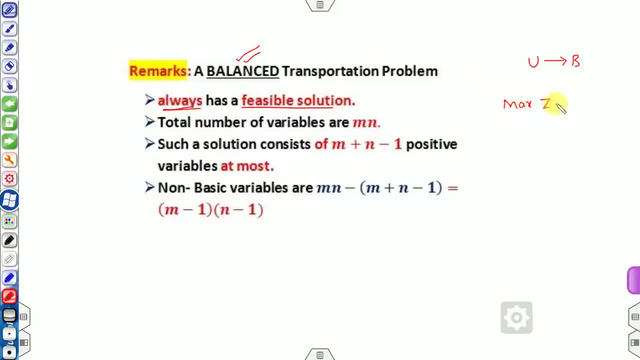 by adding a dummy from the unbalanced one, so i can convert the unbalanced transportation problem into the unbalanced. so whenever you try to convert the unbalanced transportation problem into the unbalanced transportation problem, you have to add a dummy column. according to that, whatever will you need is a dummy, and that's one way of voicing your question. this alguma. 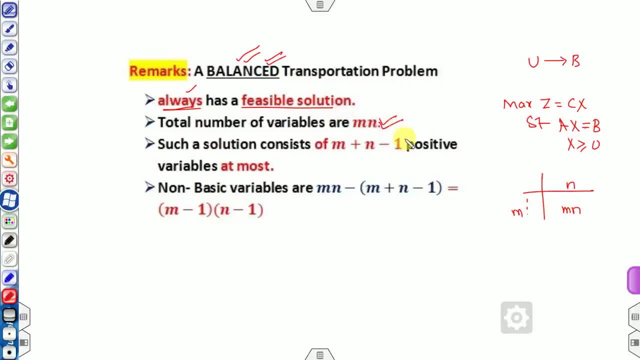 the total number of the variables are mn. okay, and out of the mn variables, such as solutions, are consisting of the m plus and positive variables at most. remember, whenever you're trying to solve the simplex method: okay, so we, we always see that the number of the basic solutions 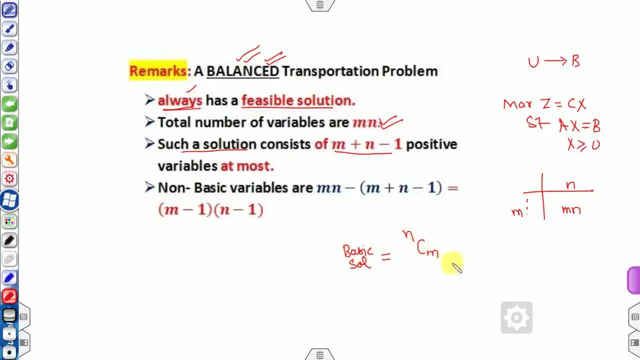 are: number of the base, ncm, okay, and the number of the non-basic solutions are. what is that? n minus mp, this is the number of the non-basic in which whose values are zero. so what is that? this is my total number of the solutions. what is the here in the transportation problem? what is the? 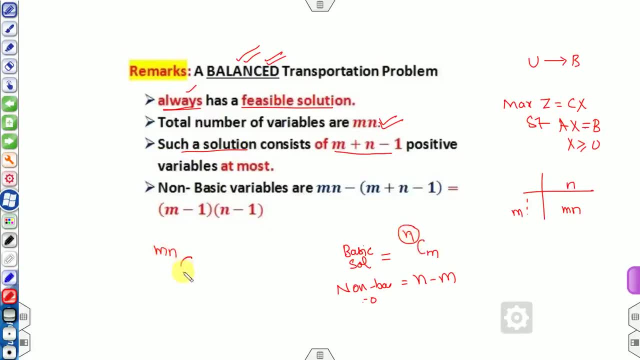 total number of the variables is mn. okay, combination. what is the m? is the rank, rank of the constraints. look at that in this here. so you call as this, sorry, xij as a ai, and second is sum is my bj, and since it is a balanced one, so what is the total number of the variables? there are the m. 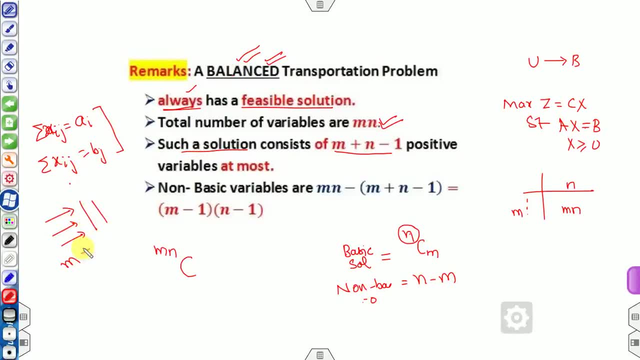 rows and there are the n columns, so total number of the constraints are this. but why we consider as a minus one because there is a one more constraint is that that is a balanced. so what is the meaning of the balance? that is, ai is nothing but the bj, so it means one additional. 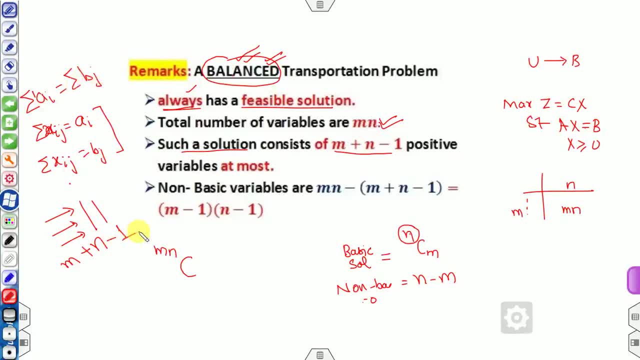 condition. so that's why m plus n minus one. what is the look at that? if i say x plus y plus z is. so what is the degree of freedom? total number of the variables are three, but you need at least the two variables in order to find the third one. okay, so it means that such a solution, consisting of the 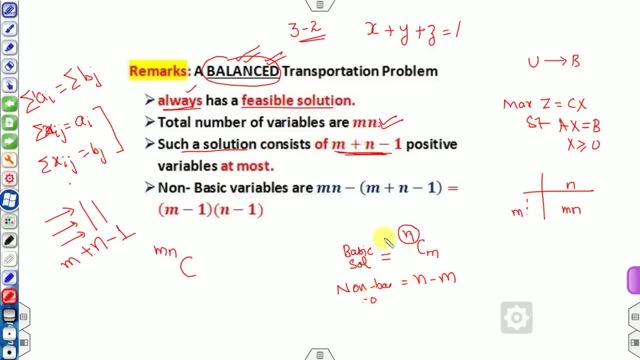 m plus n, minus one p, and the number of the non-basic variables are: and so what is the? n is total number of the variables and here. so look at that, this one is there. okay now. so these are the. these are the beautiful remarks whenever you try to solve the. 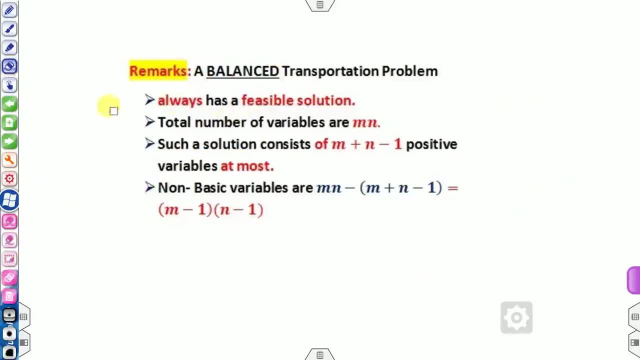 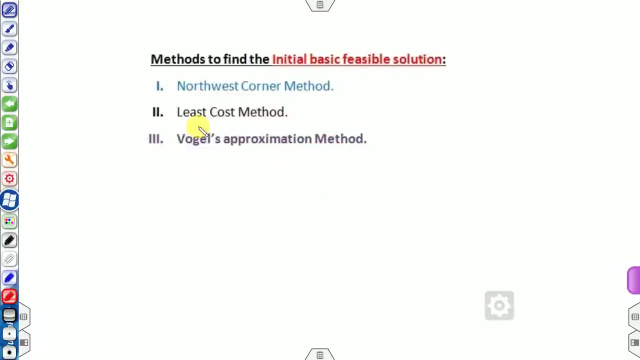 v can find the feasible solution we call as the initial feasible solution. okay, because when remember, whenever you try to solve the simplex method, you start with the s1 and s2 or s3. okay, here is 1 0, 0, 0, 1 0. okay, so these are called as the initial bfs. remember if 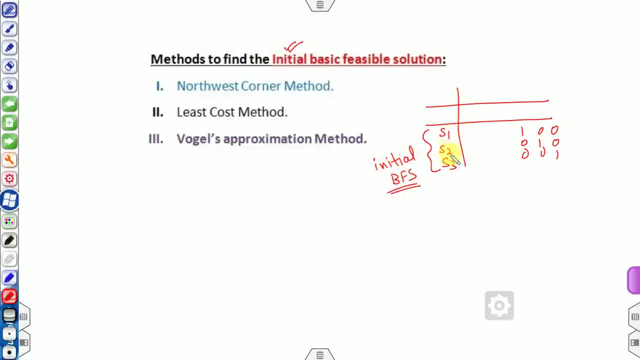 you remember the simplex method. lectures are there. so these are the initial bfs. so same for the transportation problem, how you find the initial bfs. okay, so for finding the initial bfs, there are the three methods. there are several methods are there, but generally the most important methods are three. that is, a northwest corner method, second is the least cost method and third,